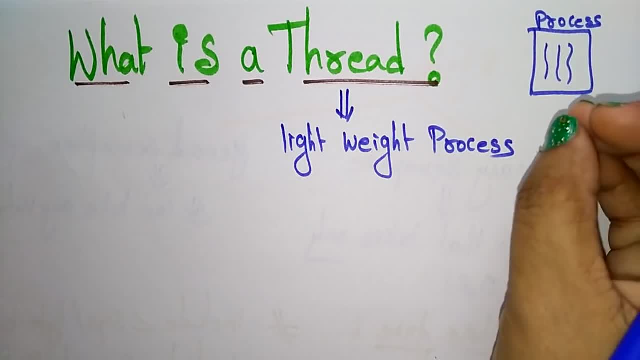 Threads means a different modules that are used. Threads are present in the process, means doing their own operation. Each process again divided into some tasks, different tasks. So that's why we call it as a lightweight process. If you take any program, so in a in that program you are having a different. you can take that like segments are different segments, or you can take the different statements So that you call it as a thread. A thread is a lightweight process. 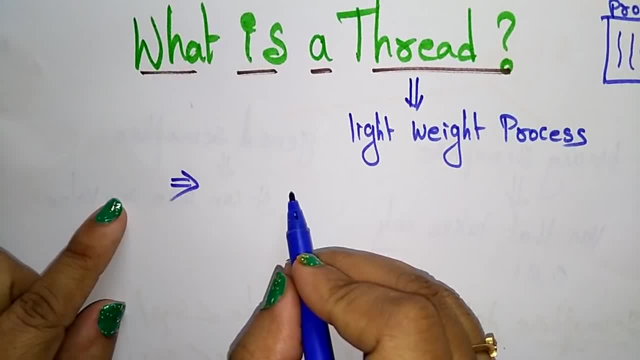 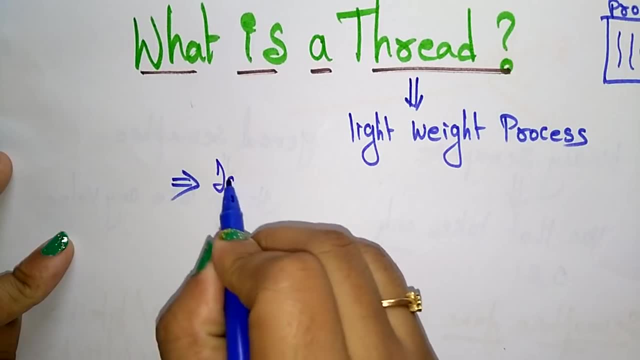 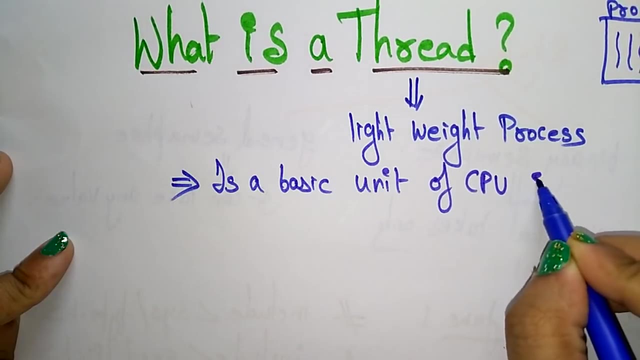 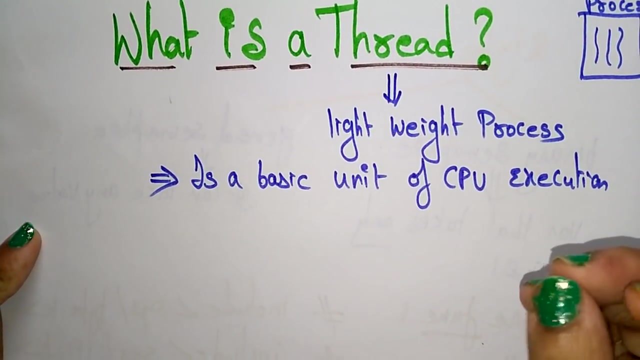 So let first me explain the definition. It is a lightweight process And it is a basic unit of a thread, is a basic unit of CPU execution. The CPU is going to be execute something so that your execution. it's a basic unit of CPU execution which, consisting of: 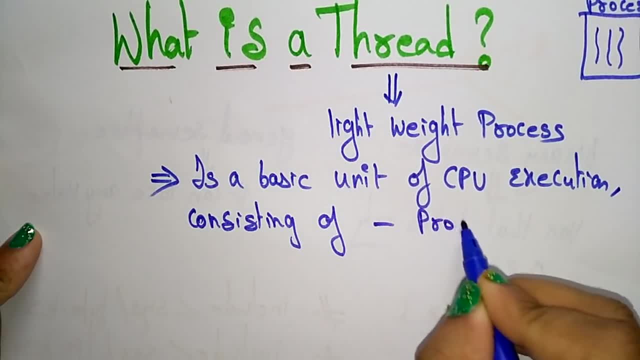 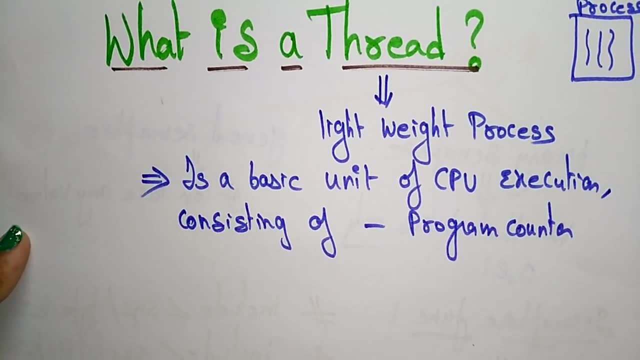 it consisting Of program counter, a thread. each thread consisting of one program counter means next, what instruction has to be executed. that information, that related address, will be stored in program counter. So each thread is having program counter and thread ID. thread ID and stack to store the temperature. to store temperature. 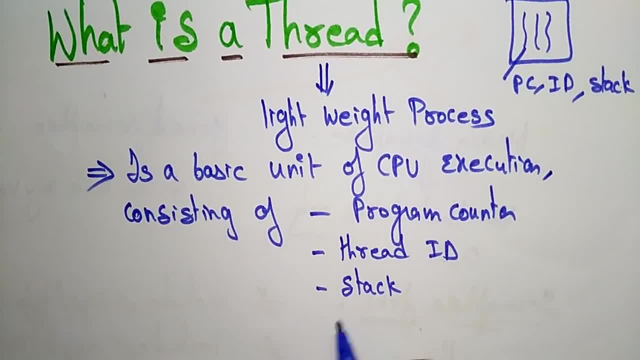 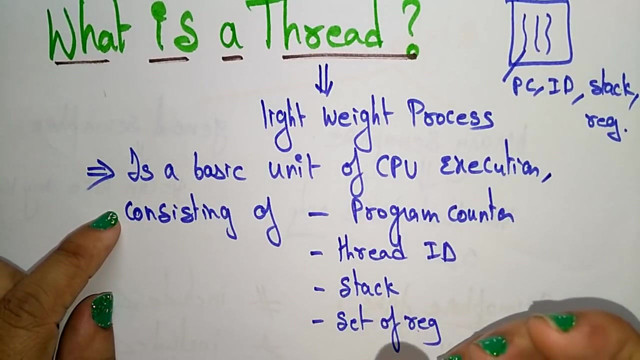 variables, you need stack And you need some set of registers- Set of registers. Okay, so that is a threat. A threat is a lightweight process. It's having a basic unit of CPU execution. the CPU is going to be execute some lightweight process, so that lightweight process is having each process here. suppose a CPU is. 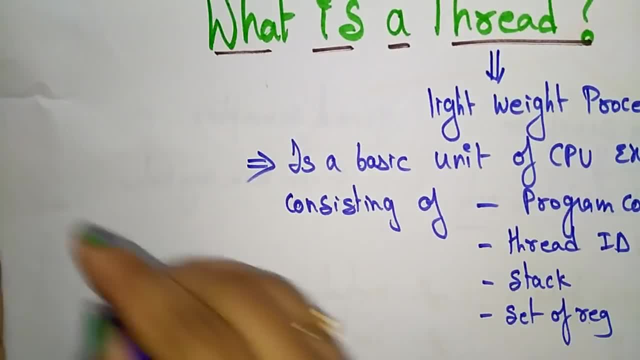 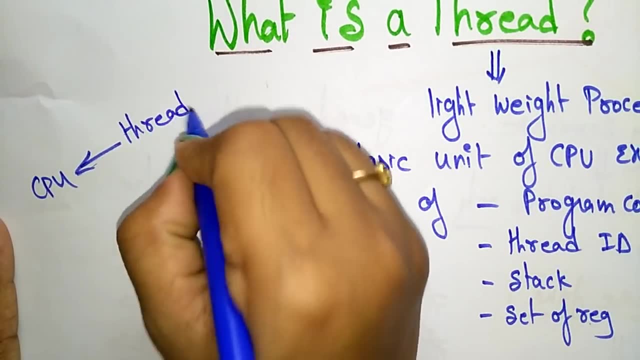 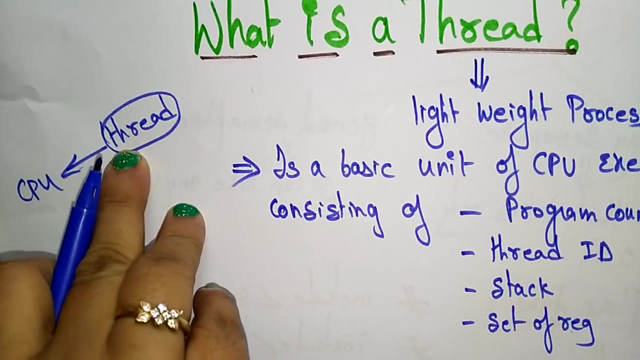 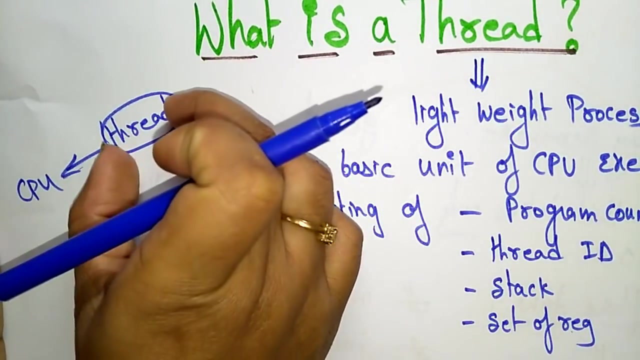 So that lightweight process is having each process Here, suppose the CPU is- is that the CPU is executing some lightweight thread? okay, so this each thread is having some program. ID, program, counter thread, ID stack and set of registers are present in each thread and that unit or basic unit is going to be executed in CPU. so actually the process is there. 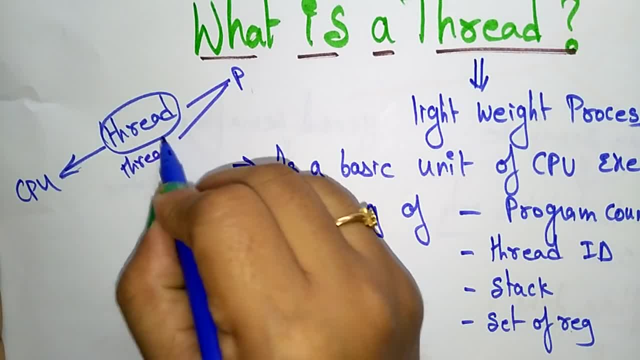 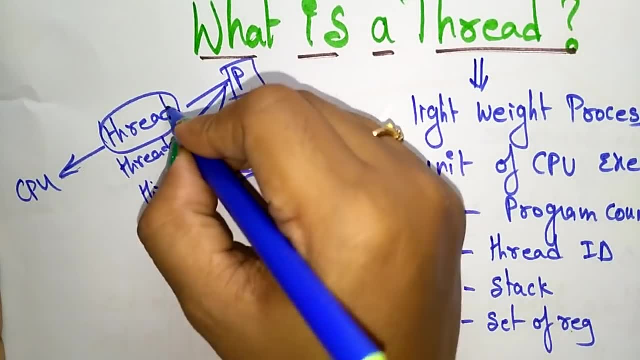 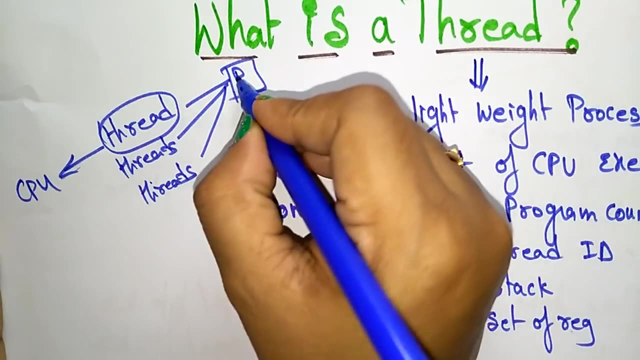 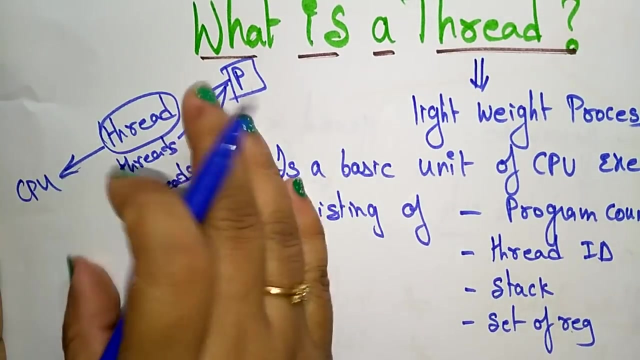 the process is having the multiple threads. that process is divided into multiple threads, each having their own function. it is doing some operation and this is doing some operation and this is doing some operation. so each operation that is doing by the process. okay, so that is having some identifications like program counter, thread ID, stack and set of registers- will be. 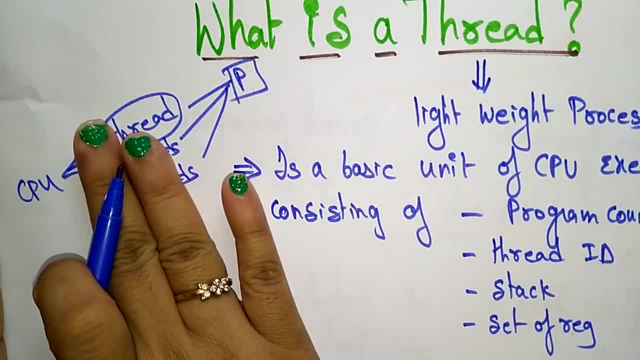 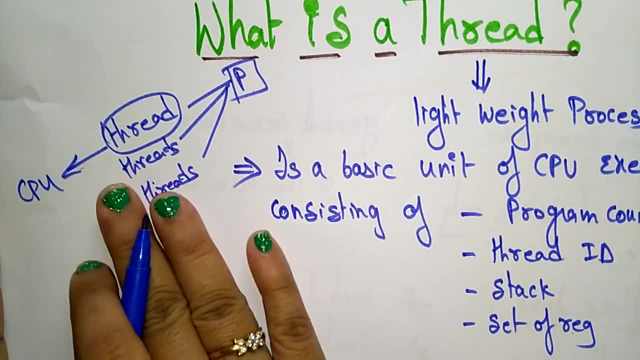 hold by each thread, so the thread will share the function like that: all the resources that are used by the process. okay, it is not an independent, so it has to share the resources of the process. it's how. it doesn't have their own resources. okay, everything will be. 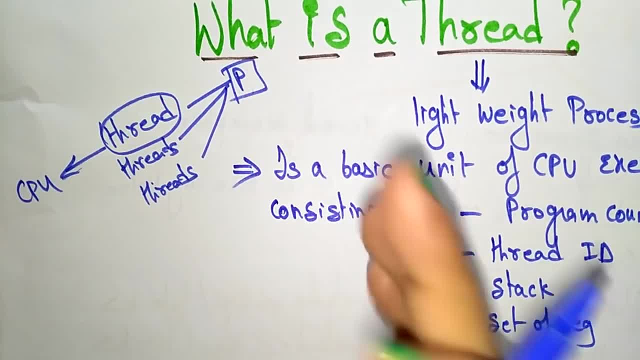 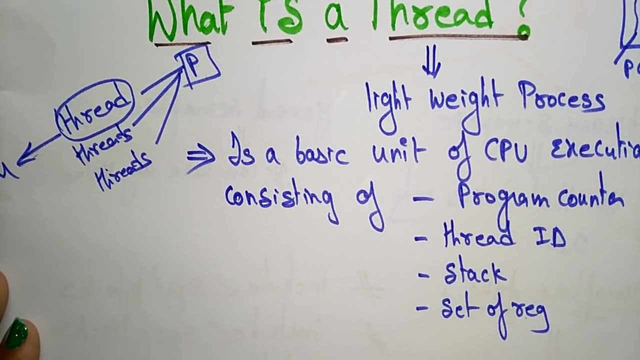 provided by the process itself. so that is a basic definition of the a thread. a thread- you call it as a thread- is a basic unit of cpu utilization consisting of program, counter, thread, id stack and set of registers that you call it as a a thread. so, however, a thread shares with other. 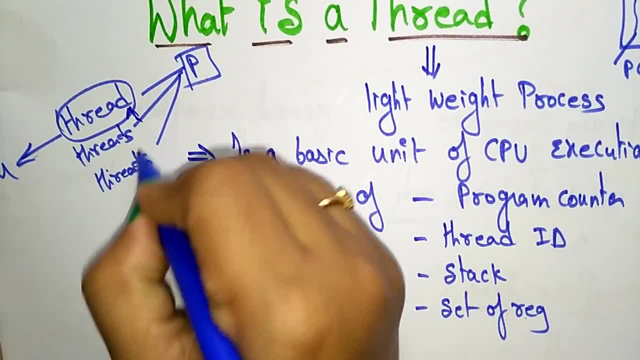 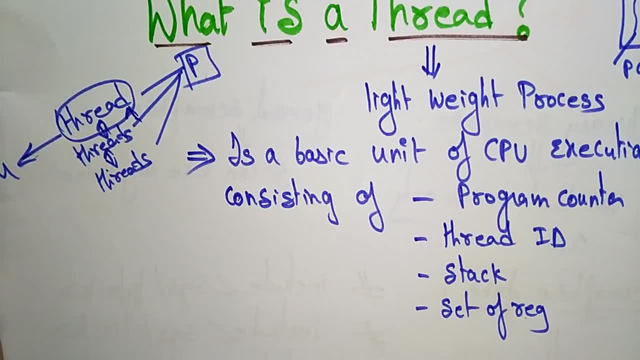 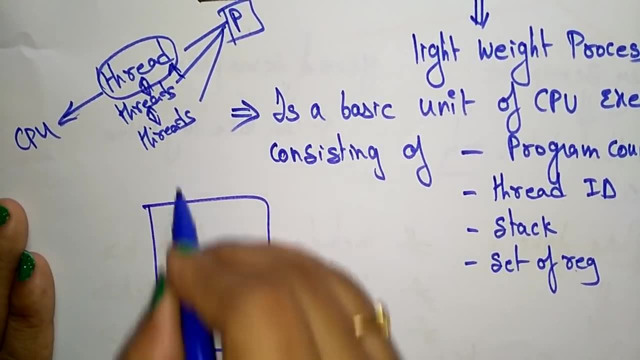 threads in the same process it shares with the other threads also. so this like this. so a thread, say, shares with the other threads in the same process its code section, data section and other operating system resources. if you take a process, the process is having some threads okay. 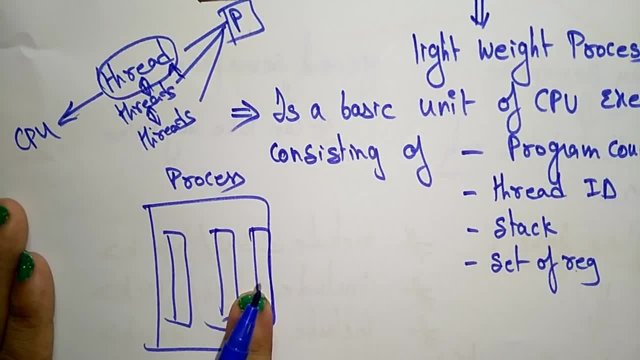 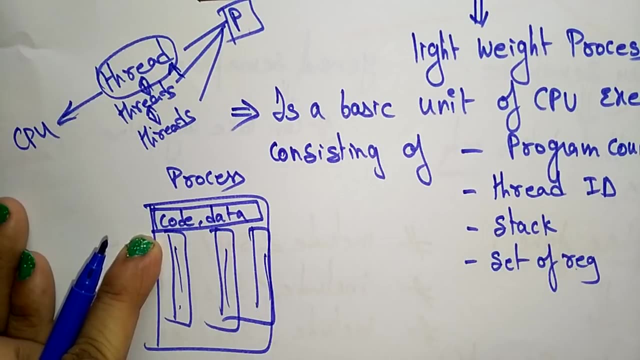 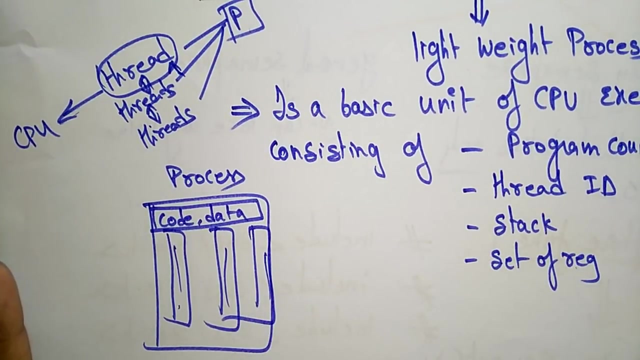 so each thread shares its code, data- everything will be shared by all threads. so all threads uses this same code and data sections and other operating system resources like files, signals- everything will be shared. so that is the concept of a process and thread. so let me give this general 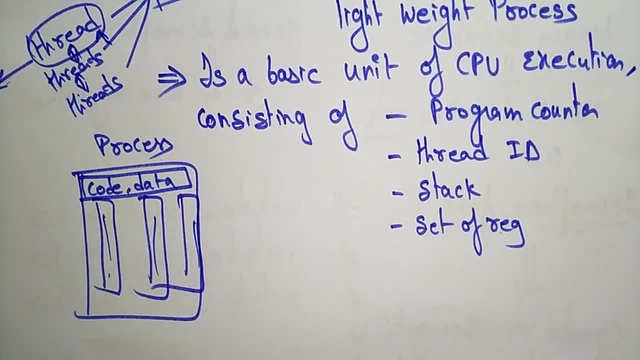 example for this process and thread. so then you will understand exactly clearly what as a process. so if you take a word, microsoft word document, if you are taken, okay, so let us take, this is a process. this is a process. so in this process you are having threads. 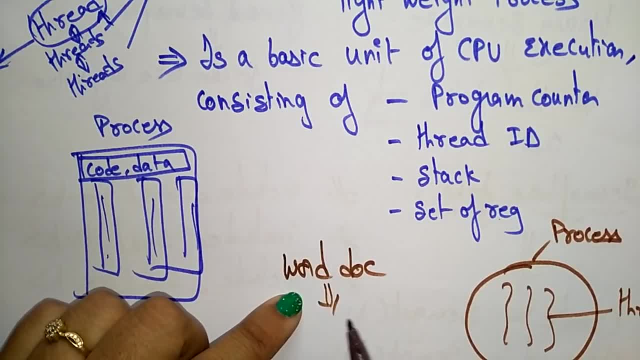 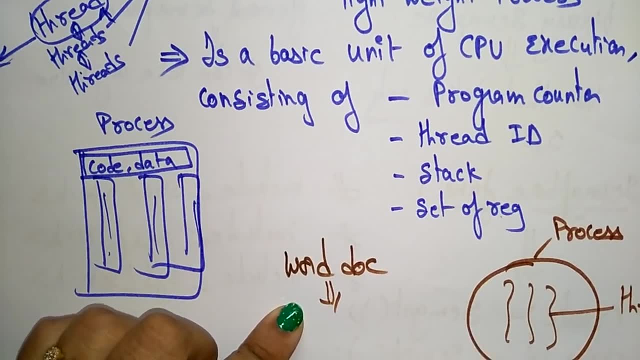 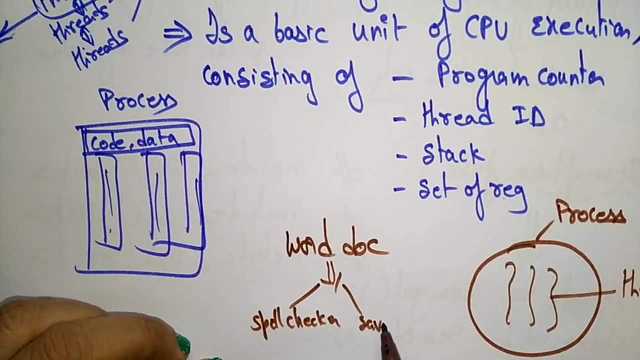 so what it means. so let us take: if you take the word document in the word document, the spell checker in a word can be considered as a thread means in the word document you are having so many features like spell checker, okay, and it is saving the files and it is. 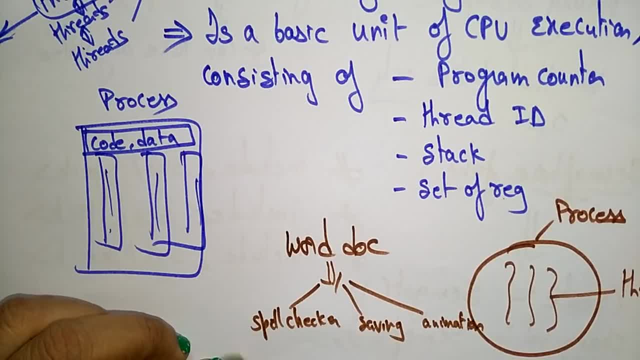 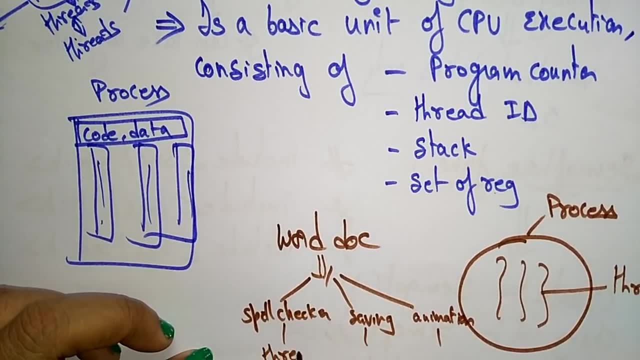 uh, creating the animations, so like this, a different uh tasks are there in the word document. so each thing you call it as a thread, it is a thread, so which is a lightweight process. so this is a process. otherwise any of these online documentation, you cancillate it. any document you should consider specifically the file which is said in tagline. in which every the blasting which you want to carry out the process, what it needs to happen is to shooting one, except even saying it in the street. something special thing is cut it and using this還 get to this shape of those areloves from which it gets see for us. So here i said, that's the texas. three pages have finished custom. 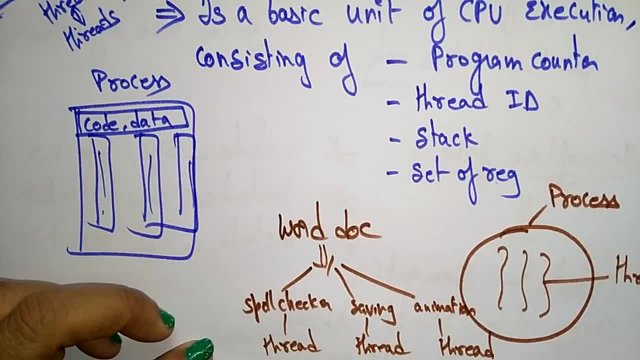 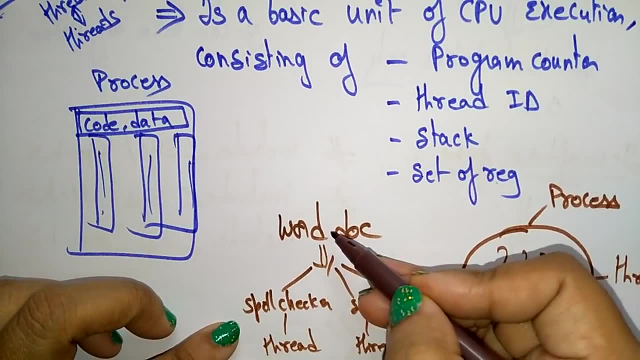 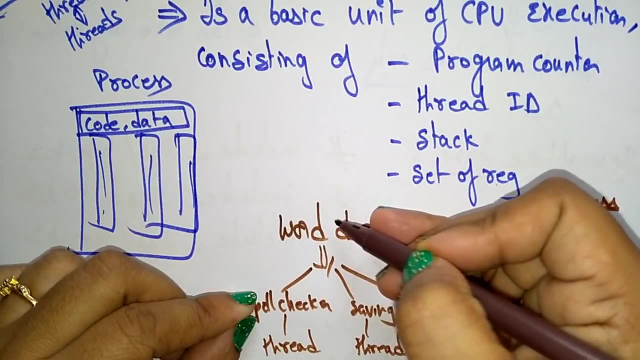 so this thread will share the resources of the word document. so the spell checkers needs the code and data and the library functions, everything that is present in the word document, so that it needs and for saving. also it needs all the code sections and the data section related in the word. 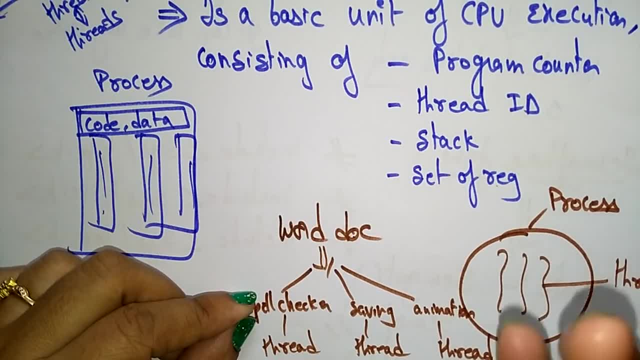 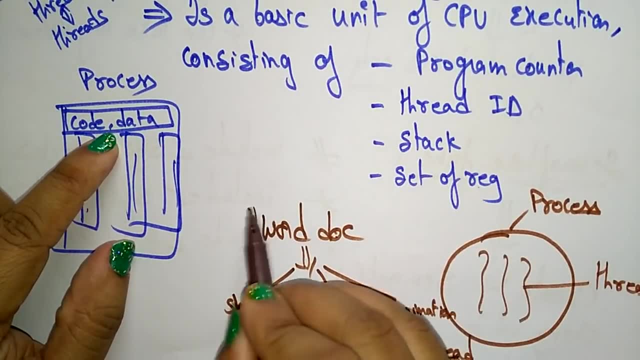 document and for creating some, any animations, or if you want to insert some picture arts. so you need the, you need to share the code and data that is present in the word document. so this is suppose, if you take, this is a process and each process, uh, for that you are having. 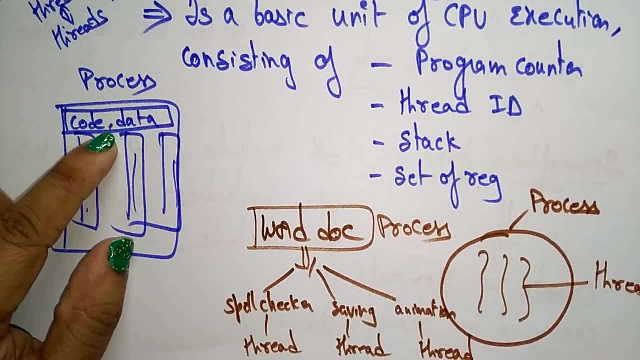 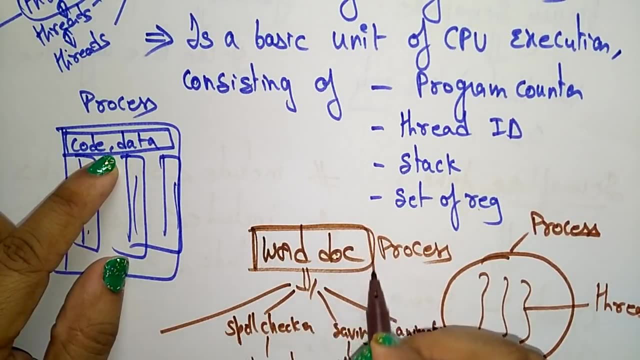 different threads: spell checkers, saving animations and coloring and, uh, whatever the operations that is there so that uniquely, uh, you call it as a thread. so an application running is called a process and application running, so this is an application. a word document is an application. you call it as a process. 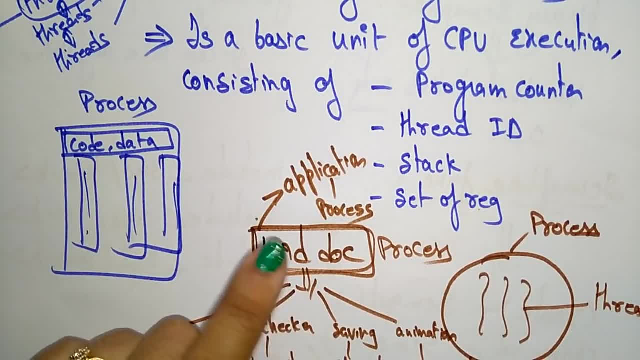 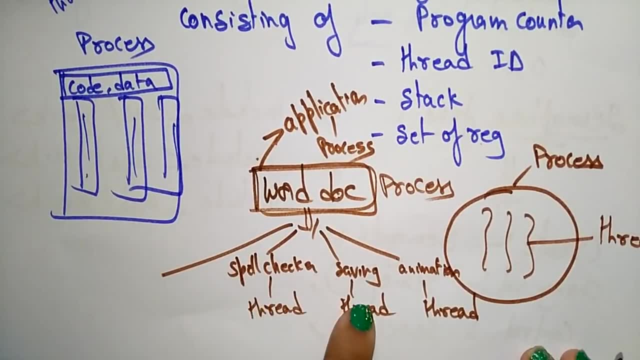 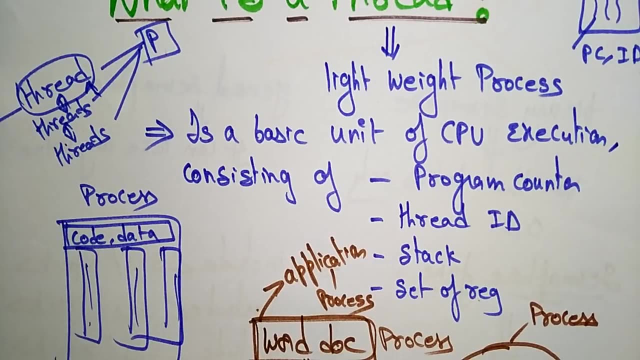 okay, so an application running is called a process, and a process can have multiple threads. a process can have multiple threads. i hope you understand, uh, the difference between this thread and the process. so a process is just and if you take an, a running application, you call it. 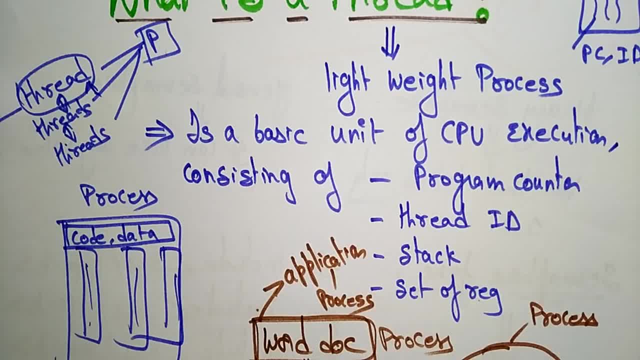 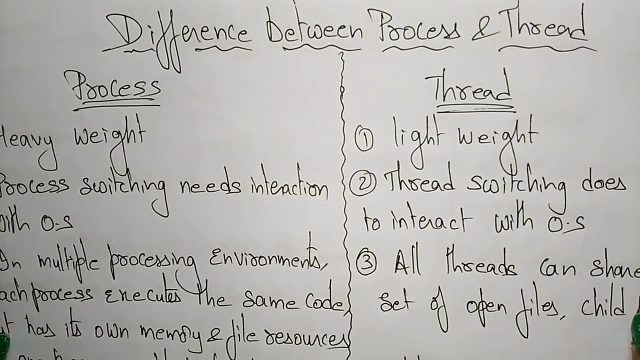 as a process and within that application, you are having different uh tasks. okay, so you can. ok, so that you call it as a threads. and now coming to this, uh, the difference between the process and thread, clearly. so let let me explain the differences between the processor and threads. 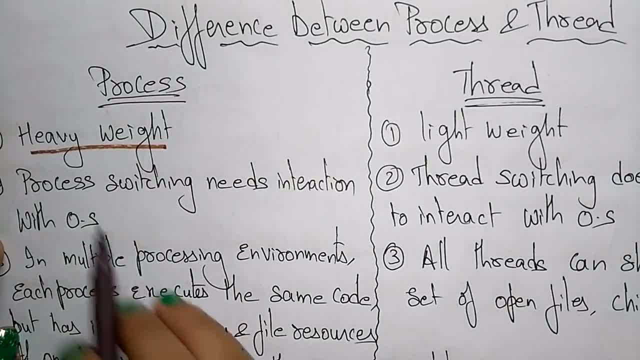 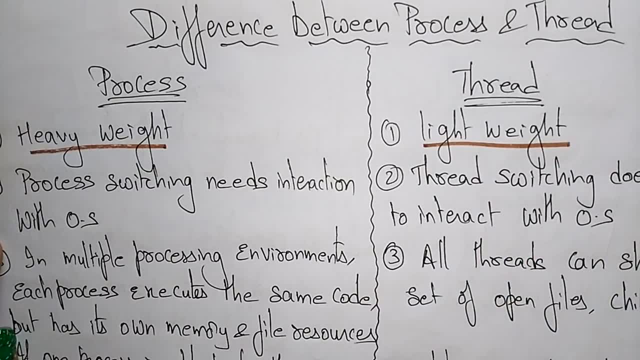 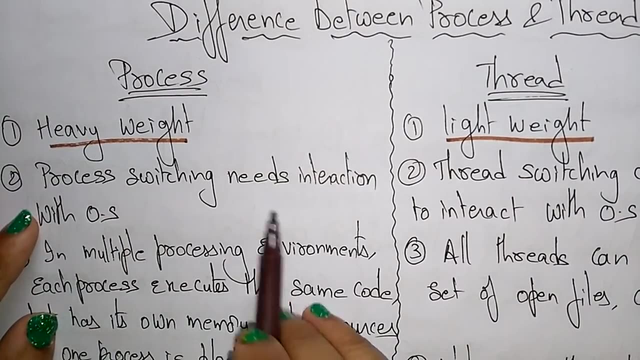 so the first, the process is the heavy weight. you call that process as a heavy weight and whereas coming to the thread, thread is a lightweight process and process switching needs. so whatever the process that you are taking, that process switching needs to be so filling. the process switching needs interaction with the operating system, so compulsory if the process wants to. 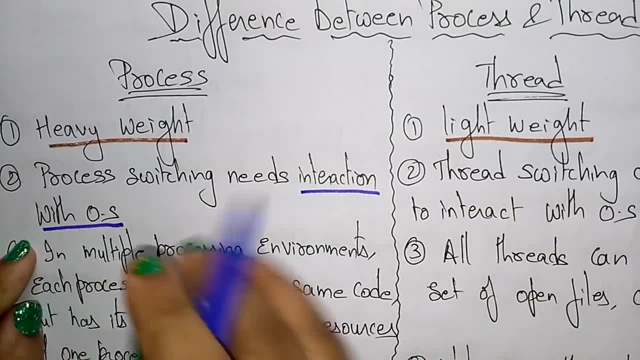 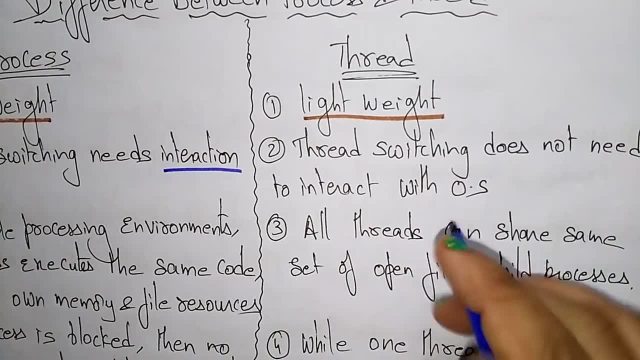 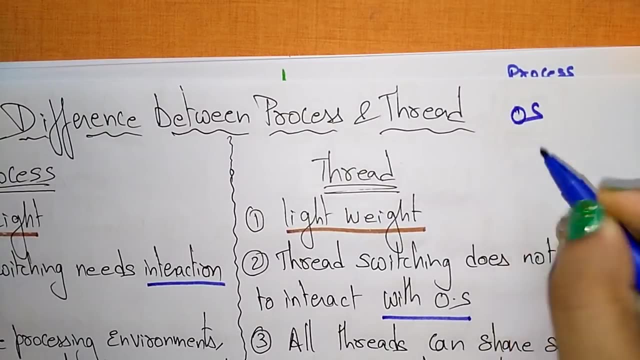 switch, it needs some interaction with the operating system. so without the interaction with the operating system the process cannot switch. but whereas coming to the thread, thread switching does not interact with operating system, so it just simply interacts with process only. okay, suppose the operating system is there. operating system is interacted with the process. 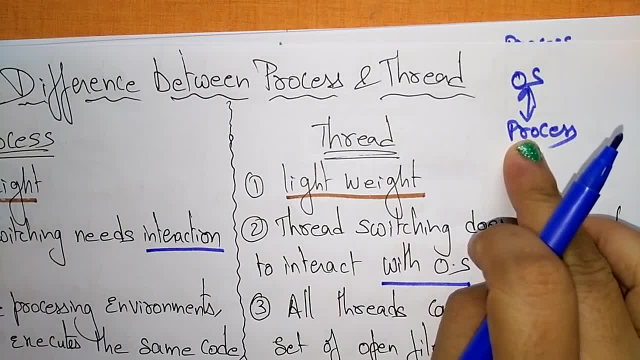 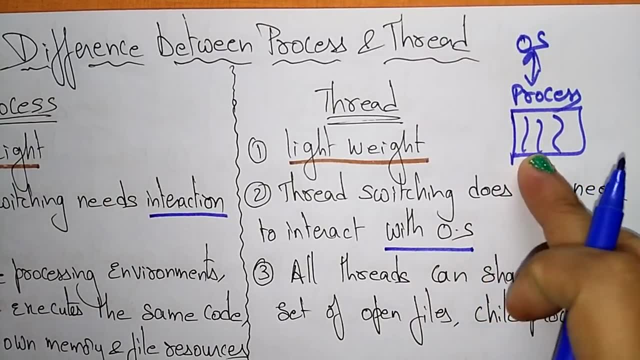 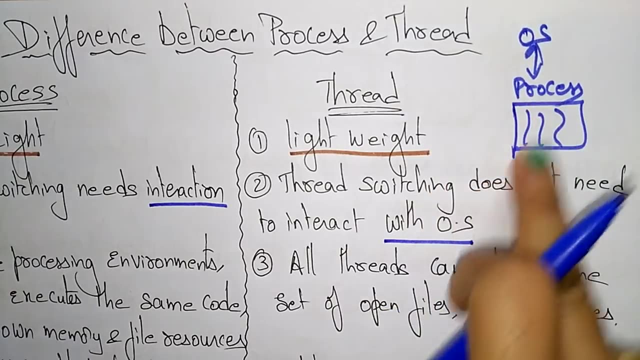 only okay. if the process wants to be switched, it needs the interaction with operating system. so within the process you are having threads. so threads no need to interact with the operating system. it just interacts with the process only because it has to share the resources of process. so it simply interacts with the process only. it doesn't interact with the operating system, does. 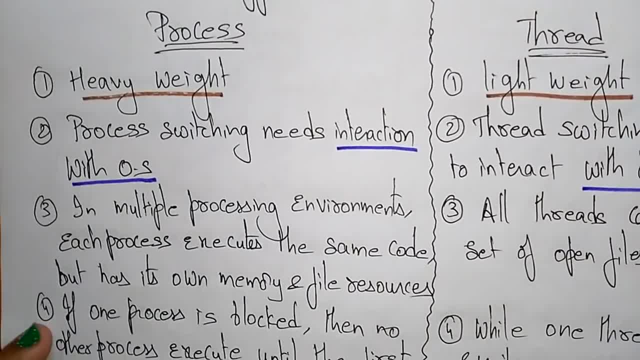 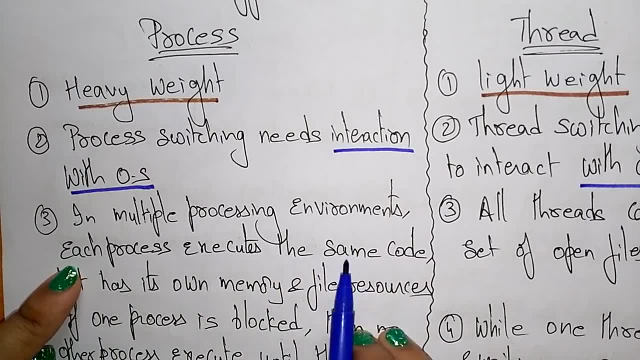 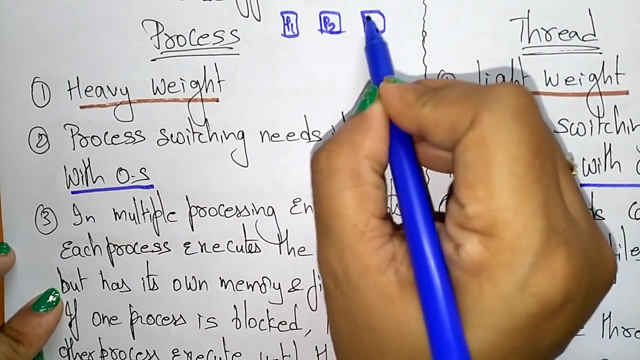 not interact with operating system next. so the process is in multi-processing and we are operating system. so the process is in multi-processing and we are operating system environment. if you take a multi-processing environment, each process execute the same code. so different process, p1, p2, p3, like the different process or the multi-processing in the 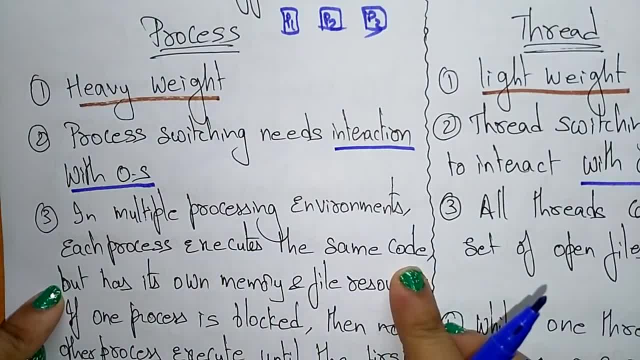 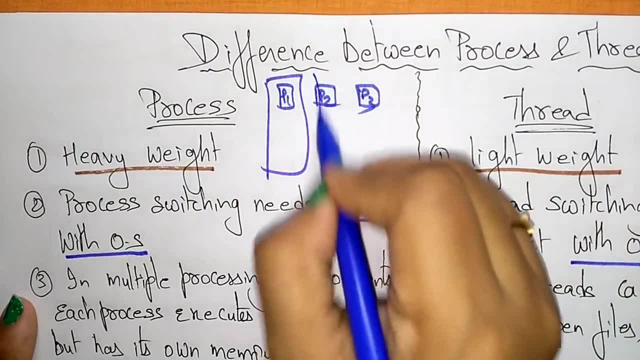 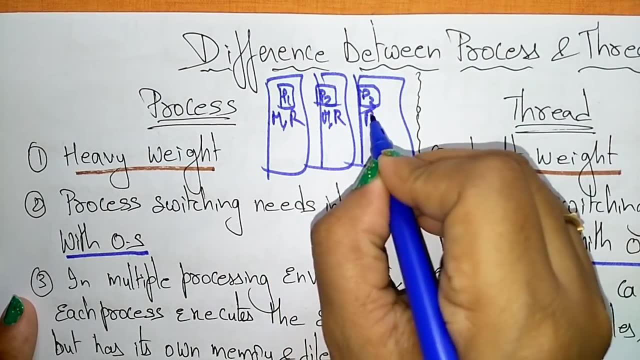 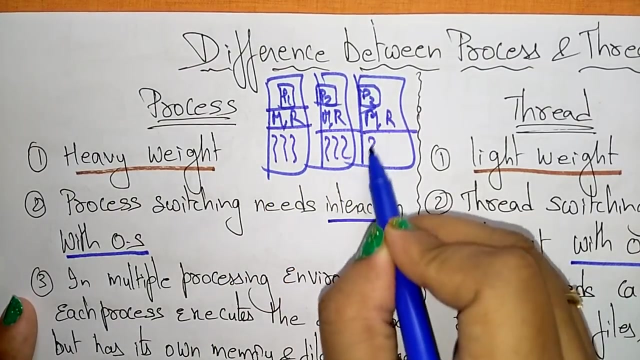 multi-processing environment. each process executes the same code but has its own memory and file resources. so each process having their own memory, own memory and the resources, file memory and the resources, file memory and the resources, file memory and the resources. okay, and this file memory and resources will be shared by multiple threads. so if you take a 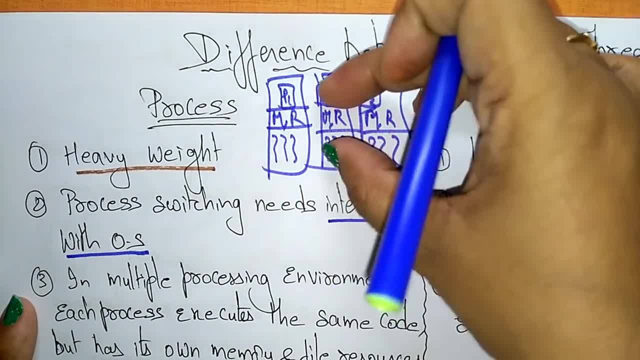 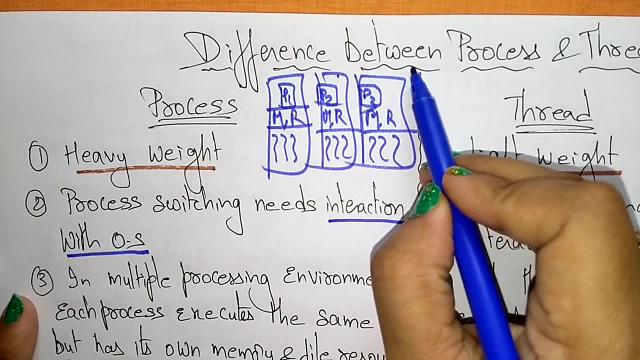 process. this process is independent of this process and this is independent of this process. so I already said, suppose, if you take the web server and if you take the database and if you take any other process, those are all independent to each other, each having their own memory and they're. 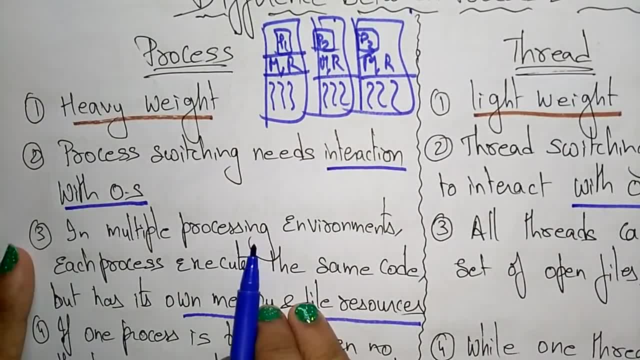 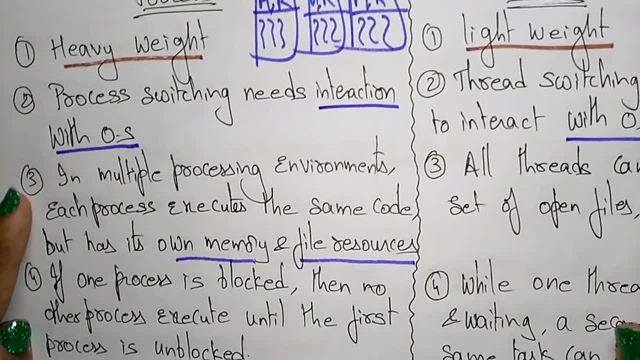 having own resources. okay, so if you take the multi-processing environment and you are operating system. so if you take a multi-processing environment, each process executes the same code but has its own memory and file resources, whereas, coming to thread, all threads can share same set of open.